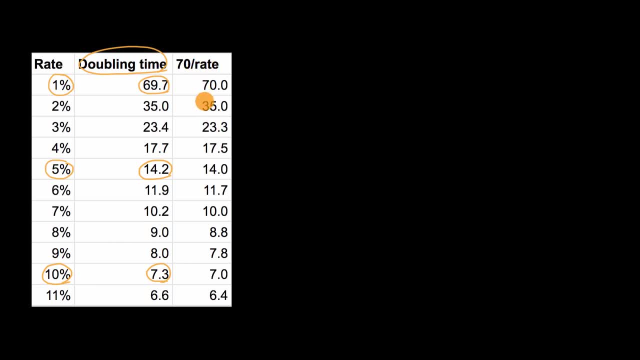 And this is known as the rule of 70. And the rule of 70 is used in a lot of different areas, a lot of different subjects. people in finance would use it because, once again, you're thinking about things growing at a certain percent every year. 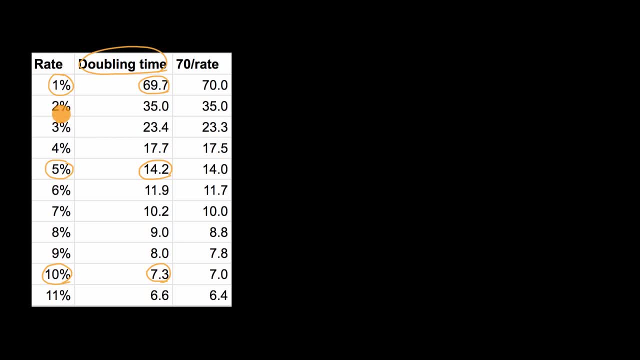 But you can also use it for things like population growth rates. So what we see with the rule of 70, and let me just write that down: rule of 70.. So what we see with the rule of 70, let me just write that down: rule of 70, and let me just write that down rule of 70.. 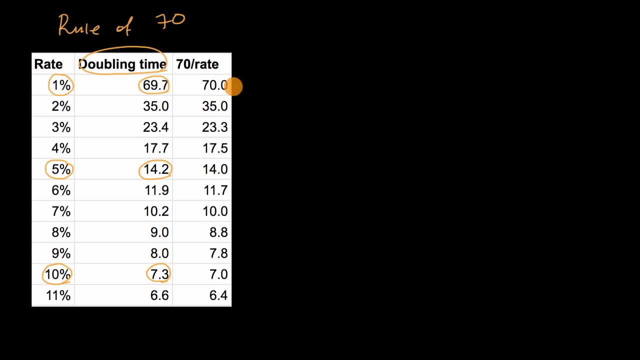 of 70 is that you can approximate the doubling time by taking the number of 70 and dividing it by the- not actually the percentage, but just the number of the percentage. So, for example, this right over here is 70 divided by this one here, which is equal to 70. 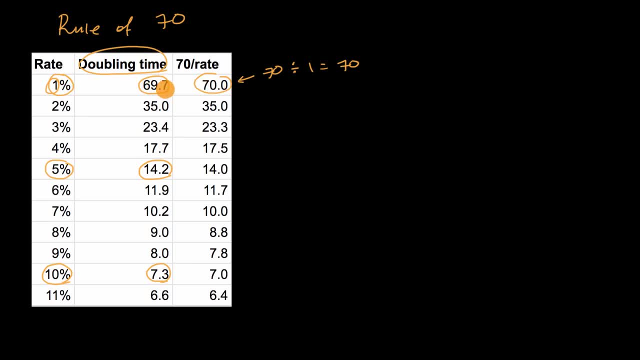 And notice this: 70 is pretty close to 69.7.. If you wanted to figure out, or you wanted to approximate the doubling time, if the population is growing at 7% a year, well, what you would say is all right. 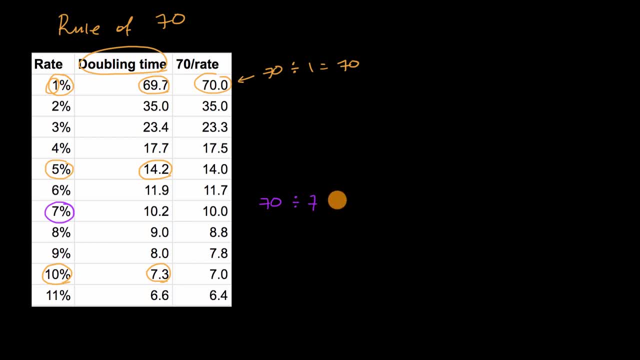 what is 70 divided by seven? Well, that is equal to 10.. So this would be your approximation, And if you were doing it in a mathematically precise way, it would be 10.2.. So if you're taking, say, an AP Environmental Science course, 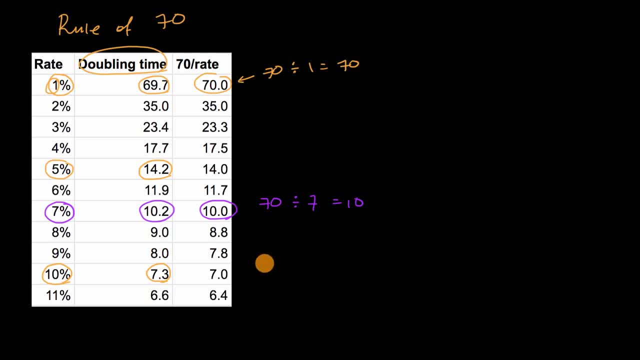 and they're asking you for how long it takes for something to double. let's say, a population that's growing 7% a year. they're probably expecting you to use the rule of 70. So let's say that we have a population. 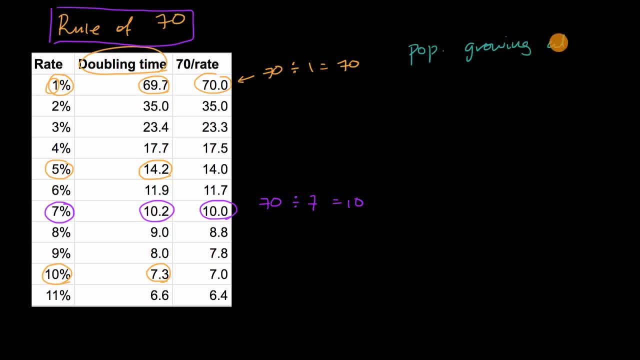 that is growing at 14% per year and that would actually be a very huge growth rate. What I want you to do is pause this video and approximate how long would it take for that population to double. All right now, let's work through this together. 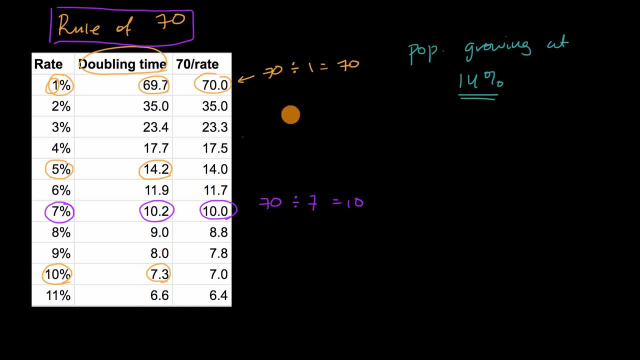 So, as I mentioned, we're approximating, We don't have to do. we calculate the exact doubling time. So if we're approximating it, it's going to be 70 divided by the rate of growth. So in this situation, 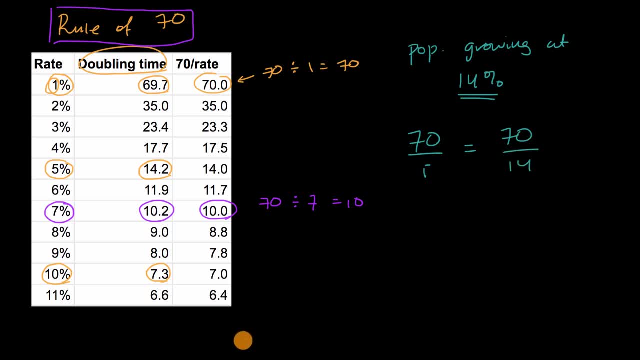 this is going to be 70 divided by 14, which is equal to five. So if a population is growing at 14%, it'll take it roughly five years to double.